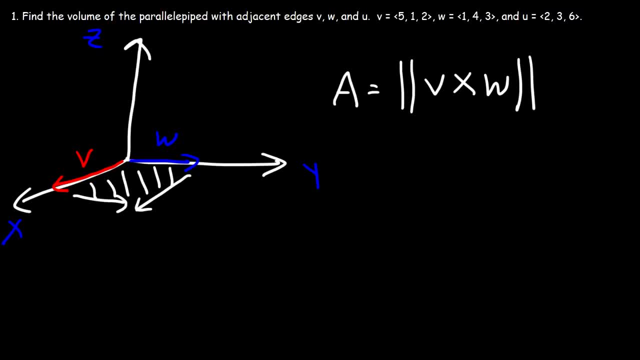 of the cross product of those two vectors. Now what we're going to do is we're going to add another vector, let's say vector U, and we're going to draw a new shape. So how can we find the volume of this parallelepiped? Notice that it's similar to the volume of 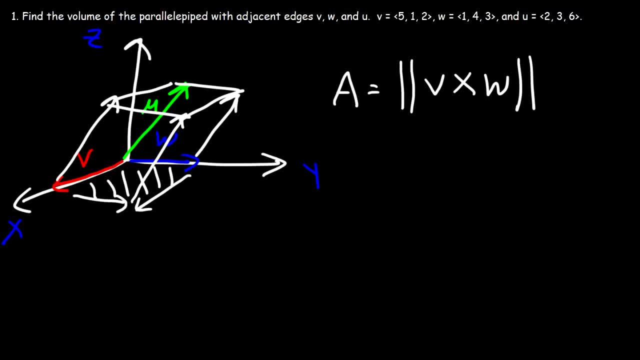 a rectangular prism. Like the shape of it looks like a rectangular prism, Though it's kind of slanted. And the volume for a rectangular prism is basically the area of the base times the height. So we have the area of the base, but we need to multiply by the height And it turns out. 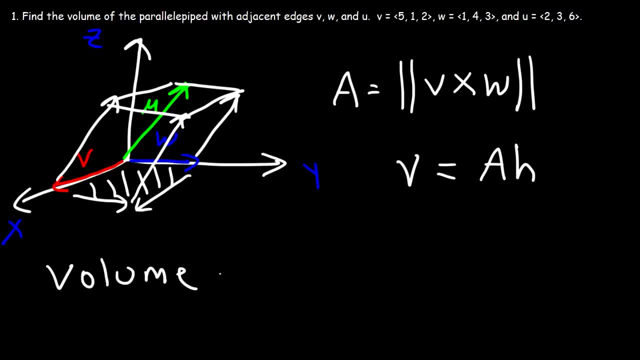 that the volume of the parallelepiped is equal to the cross product of vector U, and I mean the dot product of vector U and the cross product of vector U, V and W. so this right here is known as the triple scalar product, and that's. 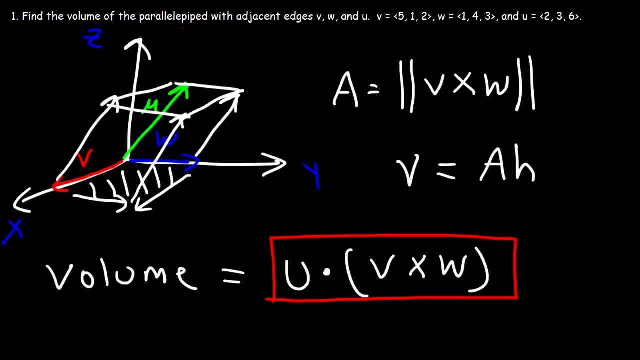 what we need to find in order to calculate the volume of the parallel pipette. so if you look at this formula, this right here tells us the area that's basically the area of the base, and vector u corresponds to the height of the parallel of pipette. so when you multiply area by height, it will give you. 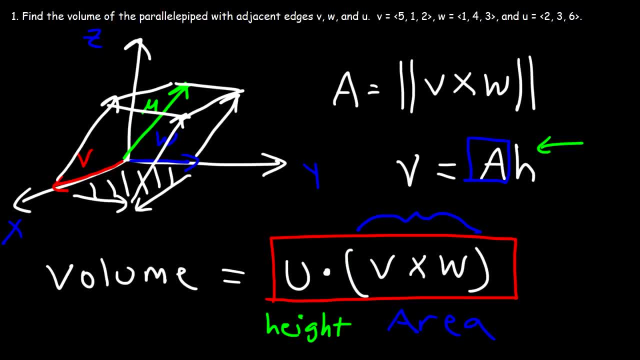 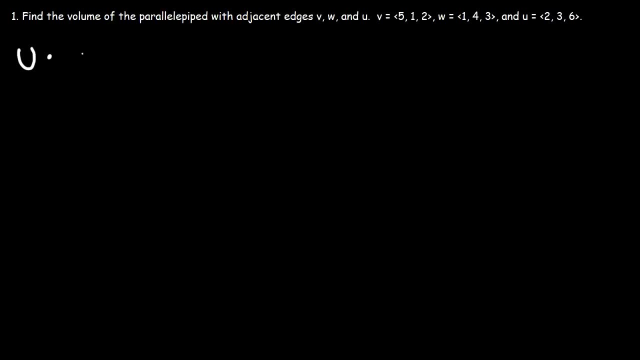 the volume. and that's just the way I think of the equation. seen it, that way makes sense to me. hopefully it makes sense to you as well. so now let's focus on this problem, let's actually let's get the answer. so how can we evaluate the triple scalar product? what 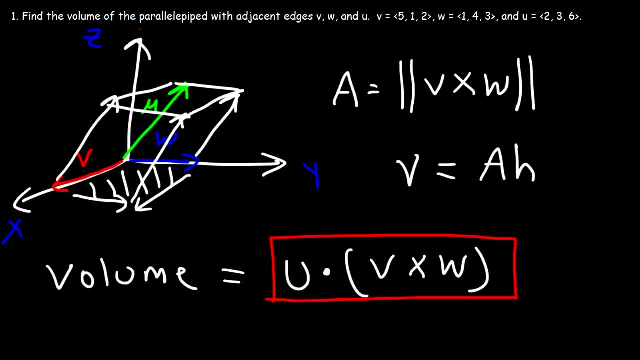 need to find in order to calculate the volume of the parallelepiped. So if you look at this formula, this right here tells us the area That's basically the area of the base, And vector U corresponds to the height Of the parallelepiped. So when you multiply area by height, it will give you. 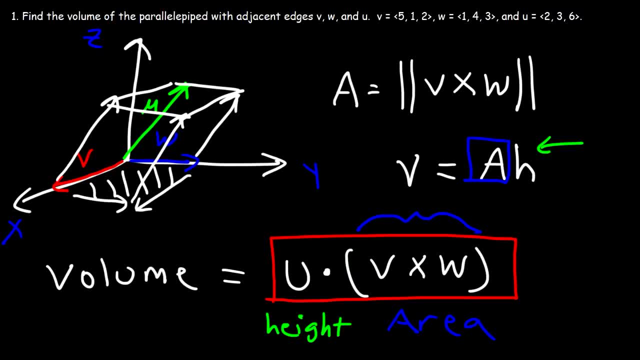 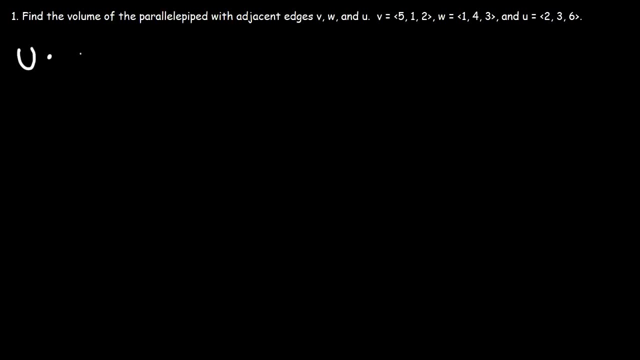 the volume, And that's just the way I think of the equation. Seeing it that way makes sense to me. Hopefully it makes sense to you as well. So now let's focus on this problem. Let's actually- let's- get the answer. So how can we evaluate the? 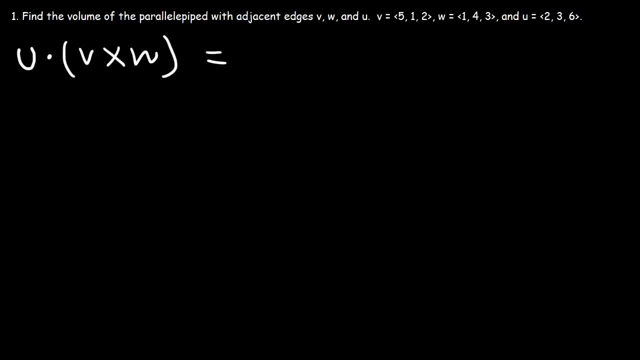 triple scalar product. What do we need to do? All we need to do is basically find the determinant of a three-by-three matrix. So first you need to write vector U in the first row and then vector V in the second row, and then vector W in the third row. So vector U. 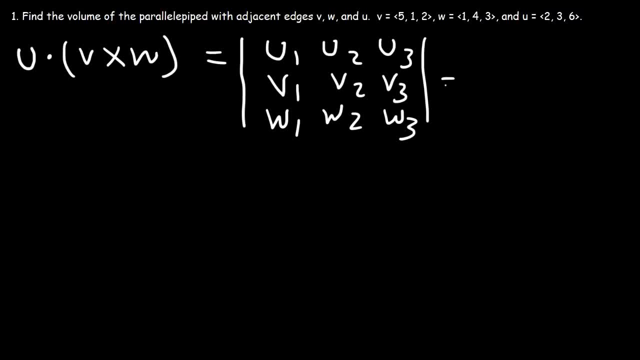 that's 2,, 3,, 6.. And then vector V: it's 5,, 1,, 2.. And then we have vector W, which is 1,, 4, 3.. Now for those of you who don't remember how to evaluate the determinant of a: 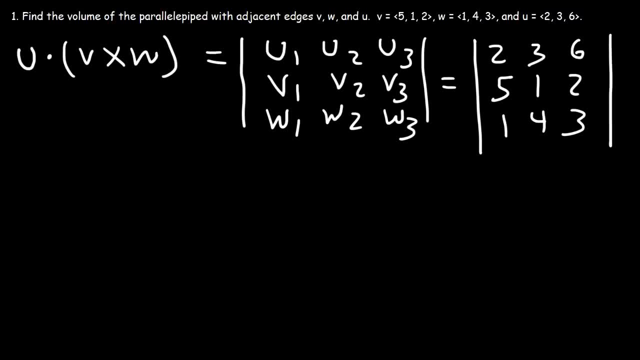 three-by-three matrix. I recommend searching out a video that I created on YouTube entitled How to Find the Determinant of a 3x3 Matrix. I just typed in Organic Chemistry Tutor. It should come up. But here's the gist of what you. 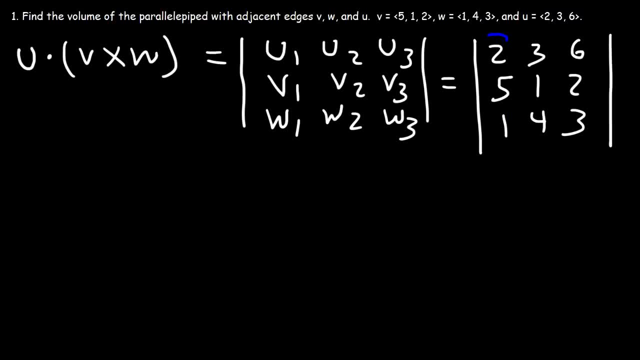 need to do So. the first thing you need to do is write the number in the first row and the first column. So we're going to write equals 2.. And then we're going to create a 2x2 matrix. So the number 2 is in the first row, first column, And 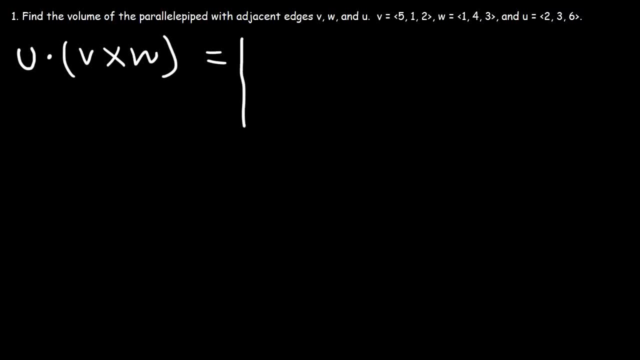 do we need to do? all we need to do is basically find the determinant of a three-by-three matrix. so first you need to write vector u in the first row and then vector V in the second row and then vector W in the third row. so vector u, that's two, three, six, and then vector V, it's five. 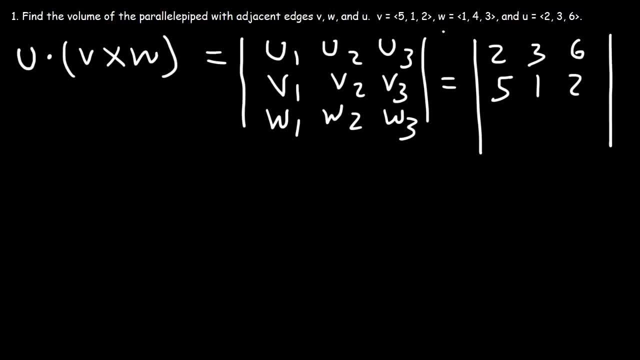 one, two, and then we have vector W, which is one, four, three. now, for those of you who don't remember how to evaluate the determinant of a triple scalar product of a three-by-three matrix, I recommend searching out a video that I created on YouTube entitled how to find the determinant with three by three matrix. 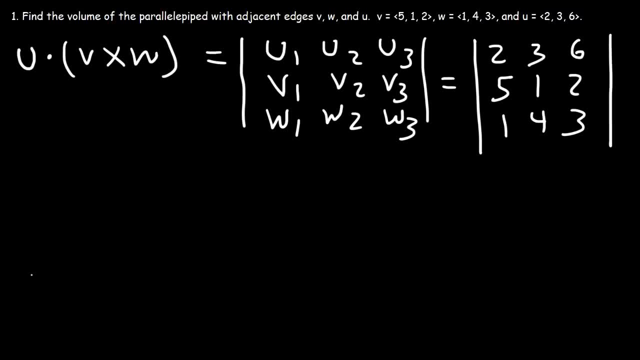 and just type in organic chemistry tutor should come up. but here's the gist of what you need to do. so the first thing you need to do is write the number in the first row and the first column. so we're gonna write equals two and then we're going to create a two by two matrix. so the number two is in the 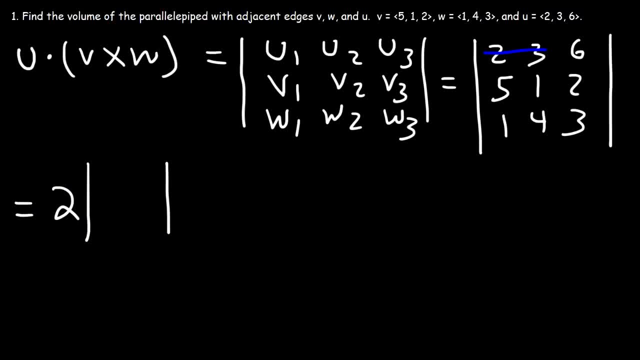 first row and the first row, first column, and notice that it leaves behind these four numbers, which is what we're going to put in our two by two matrix. so we have one, two, four, three, and then it's going to be minus the second number in the first row, which is three, and that number is in the first row, second column. 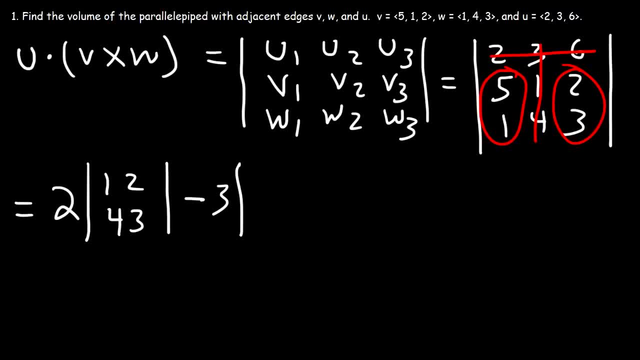 so it leaves behind the numbers five, one, two, three. so let's put five, one, two, three inside this matrix and then plus the last number in the first row, which is six, and that's in the first row, third column. so it leaves behind the numbers five, one, one, four. as you can see here now the 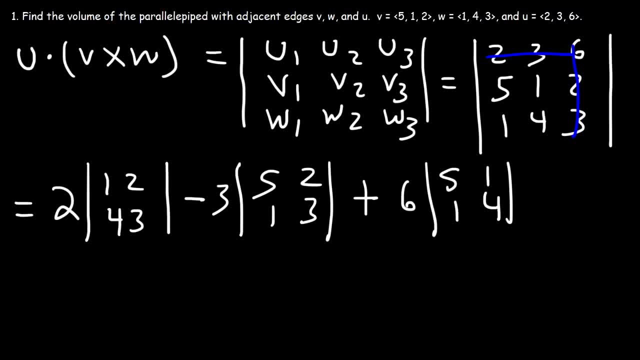 last thing that we need to do is we need to evaluate the determinant of a two by two matrix. so let's say, if we have the matrix ABCD, it's going to be a times D minus B times C. so that's what we're going to. 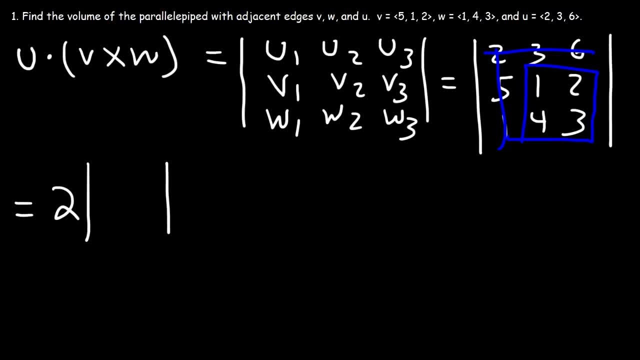 notice that it leaves behind these four numbers, Which is what we're going to put in our 2x2 matrix. So we have 1,, 2,, 4,, 3.. And then it's going to be minus the second number in the first row, which is 3.. And 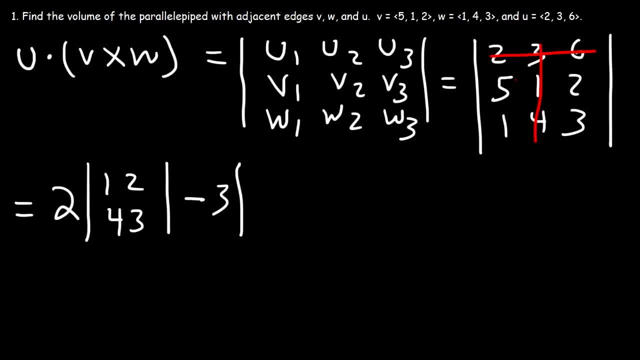 that number is in the first row, second column, So it leaves behind the numbers 5, 1,, 2, 3.. So let's put 5, 1,, 2, 3 inside this matrix And then plus the last number in. 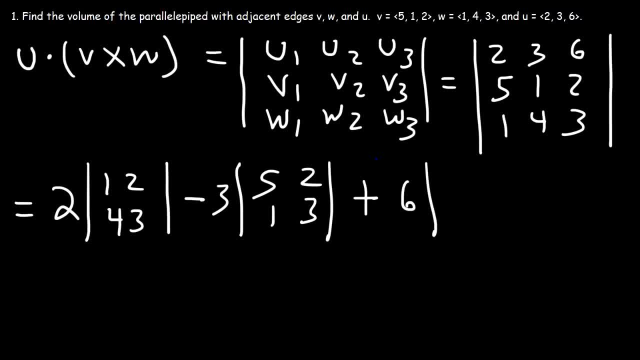 the first row, which is 6, 2, 3.. And that's in the first row, third column. So it leaves behind the numbers 5, 1, 1, 4.. As you can see here, Now, the last thing that we need to do is we need to. 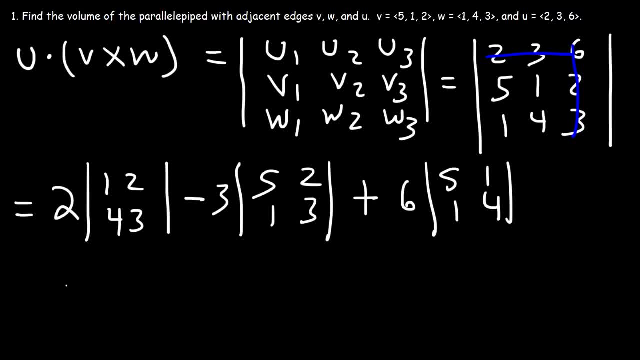 evaluate the determinant of a 2x2 matrix. So let's say, if we have the matrix ABCD, It's going to be A times D minus B times C. So that's what we're going to do next To evaluate these three 2x2 matrices. 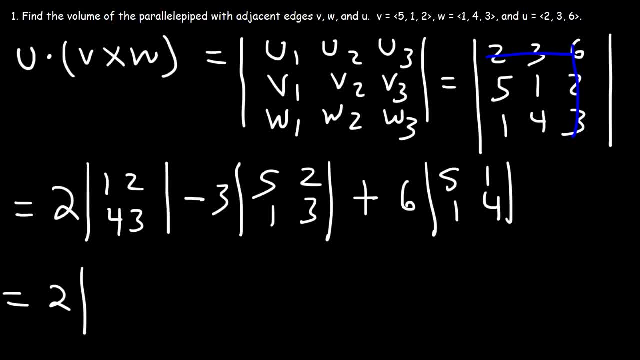 So it's going to be 3 times 1,, which is 3.. And then minus 4 times 2,, which is 8.. And then minus 3.. 5 times 3 is 15.. Minus 1 times 2,, which is 2.. 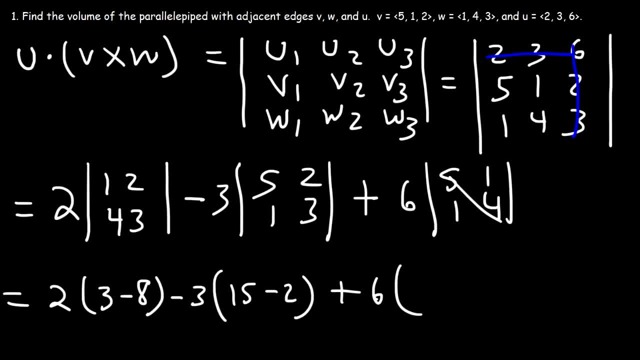 and then plus 6, 5 times 4 is 20, minus 1 times 1,, which is 1.. 3 minus 8 is negative, 5, 15 minus 2 is 13, and 20 minus 1 is 19.. 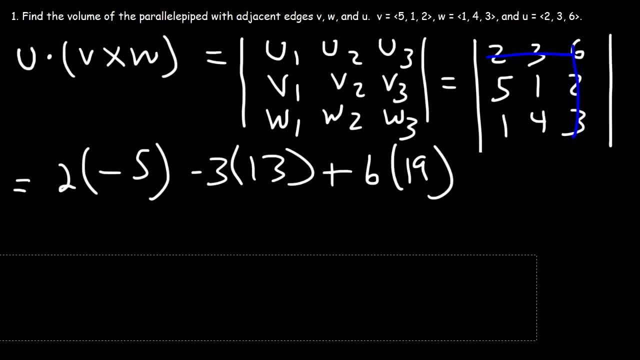 Now 2 times negative 5, that's negative 10, 3 times 13 is 39,. 6 times 19,. 6 times 20 is 120,. 6 times 1 is 6,, so 120 minus 6, that's 114.. 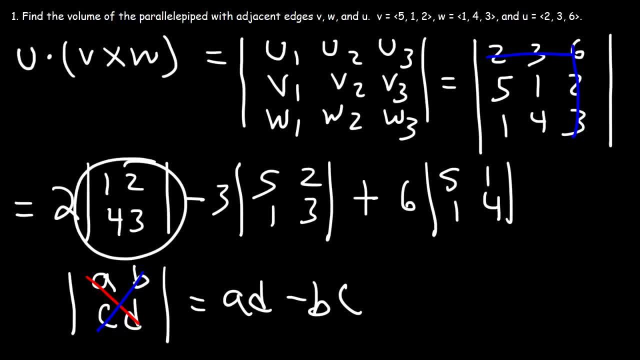 do next to evaluate these three two by two matrices. so it's going to be three times one, which is three, and then minus 4 times 2, which is 8, and then minus 3: 5 times 3 is 15 minus 1 times 2, which is 2, and then plus 6: 5 times 4 is 20 minus 1 times 1, which is 1. 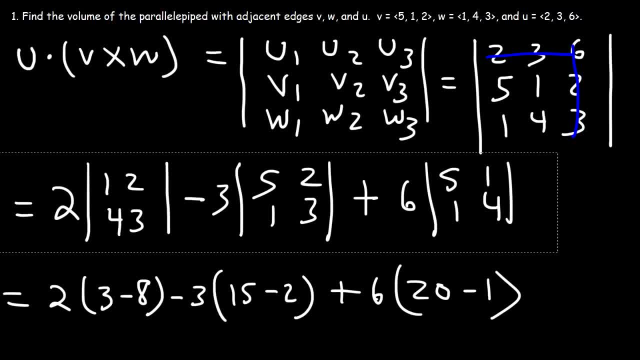 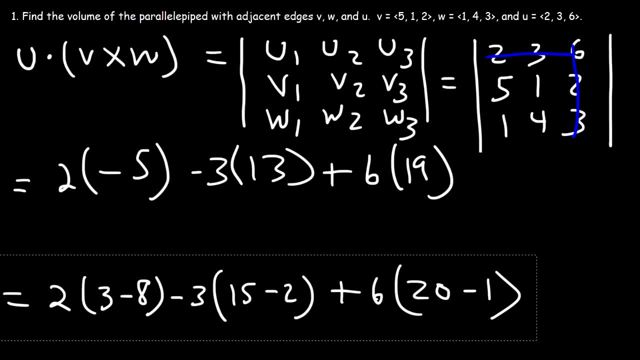 3 minus 8 is negative. 5, 15 minus 2 is 13 and 20 minus 1 is nineteen. now two times negative: 5, that's negative. 10 three times 13 is 39, six times nineteen. six times twenty is 120, six times 1 is: 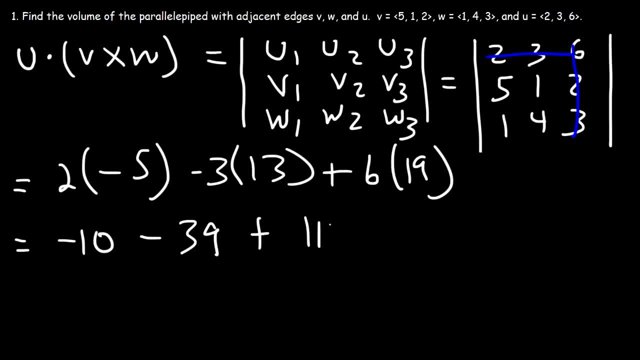 6. so 120 minus 6, that's 114. so now we gotta add these three numbers: negative 10 plus negative 39 plus 114.. That gives us 65.. So this is the volume of the parallelepiped in cubic units. 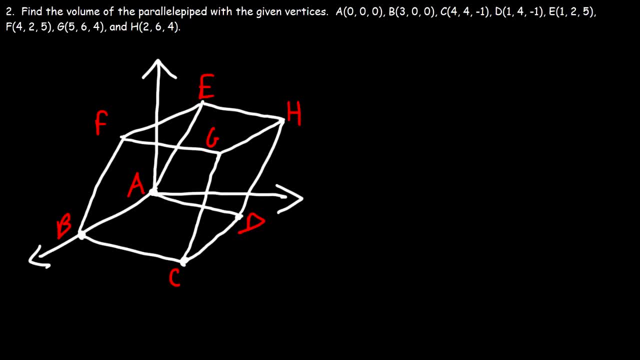 So this is the answer. Now let's move on to the next problem: Find the volume of the parallelepiped with the given vertices. So how should we do it? In this case, just like before, we need to take the information that we're given and somehow get three vectors that form adjacent edges. 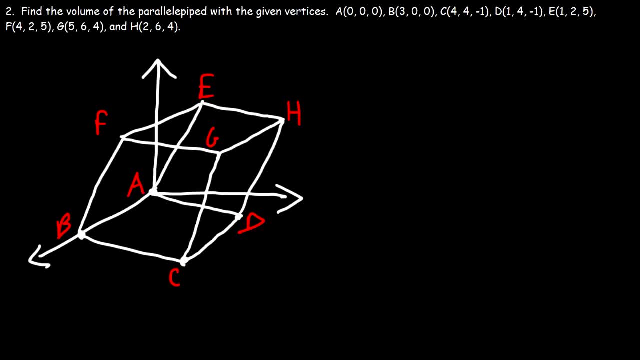 on the parallelepiped, And the best way to do that is to find basically a starting point, In this case point A, because that's the origin. And so we're going to draw our three vectors starting from point A. So we're going to say the first one is, let's call it vector V, So that's. 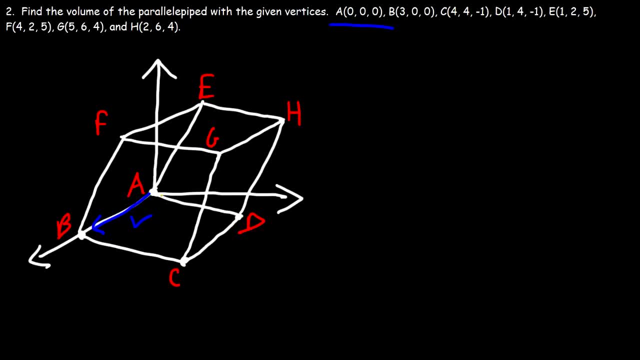 going from A to B. The second one going from A to D, let's call that vector W. And the last one, A to E, we'll call it a vector U. So those are the three vectors that form adjacent edges on the parallelepiped. 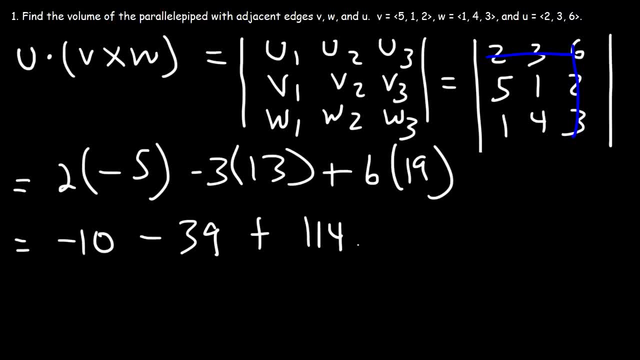 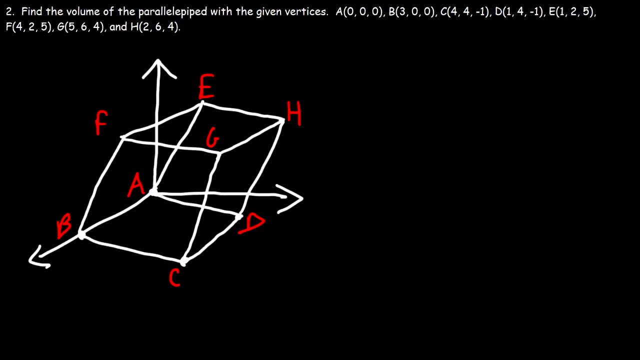 So now we gotta add these three numbers: negative 10 plus negative 39 plus 114, that gives us 65.. So this is the volume of the parallelepiped in cubic units. So this is the answer. Now let's move on to the next problem. Find the volume of the parallelepiped with the given vertices. 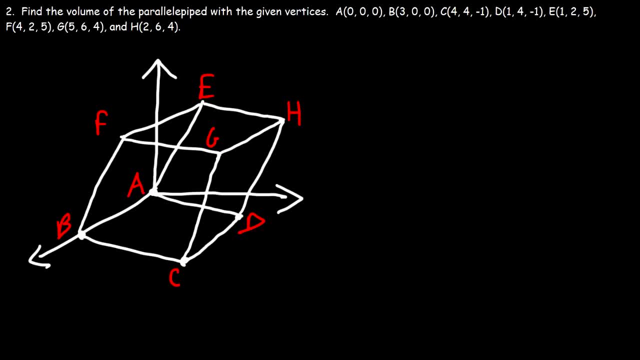 So how should we do it In this case? just like before, we need to take the information that we're given and somehow get three vectors that form adjacent edges on the parallelepiped, And the best way to do that is to find, basically a starting point, In this case point A, because that's the origin. 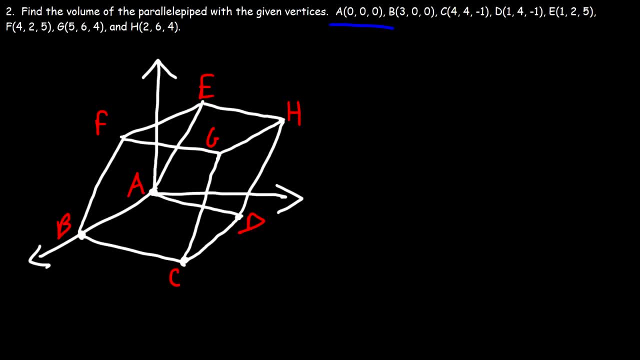 And so we're gonna draw our three vectors, starting from point A. So we're gonna say: the first one is: let's call it vector V, so that's going from A to B. The second one, going from A to D, let's call that vector W. 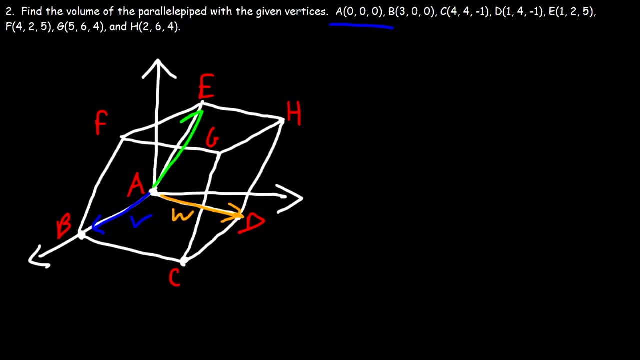 And the last one, A to E, we'll call it vector U. So those are the three vectors that form adjacent edges on the parallelepiped. Now let's start with the first vector, vector V. So vector V is basically the same as vector A, B. 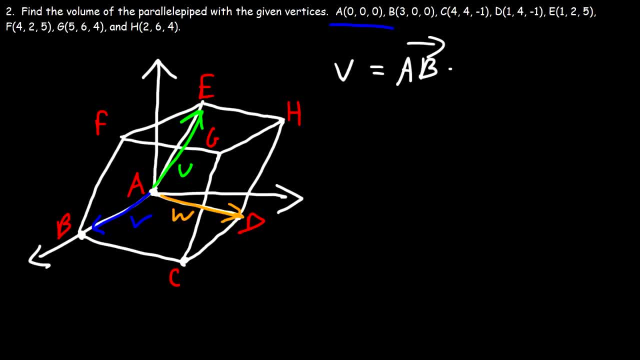 because it starts at wall point. So as it goes up it stays at wall point from A and it points towards B. Now if we take the difference between points B and A, if you subtract B minus A, you're going to get the vector 3, 0, 0.. Next we have a vector 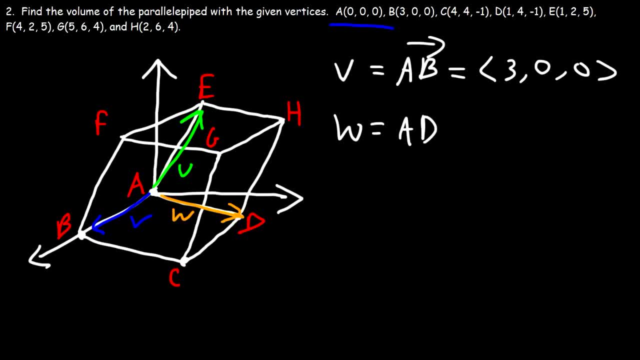 W, which starts from A and points towards D, And so if we subtract D from A, it's just going to be the same as point D, So we get the vector 1,, 4,, negative 1.. And the last: 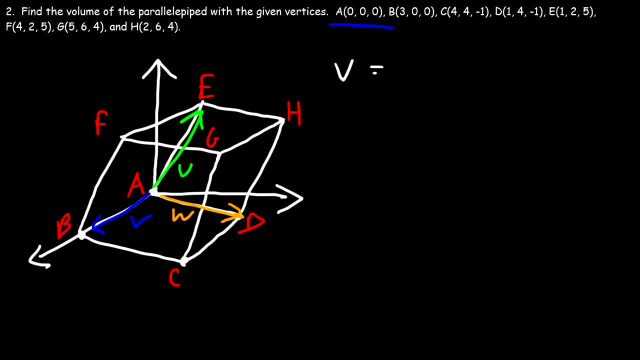 Now let's start with the first vector, vector V. So vector V is basically the same as vector AB, because it starts from A and it points towards B. Now, if we take the difference between points B and A, if you subtract B minus A, you're going to get the vector 3, 0, 0.. Next we have 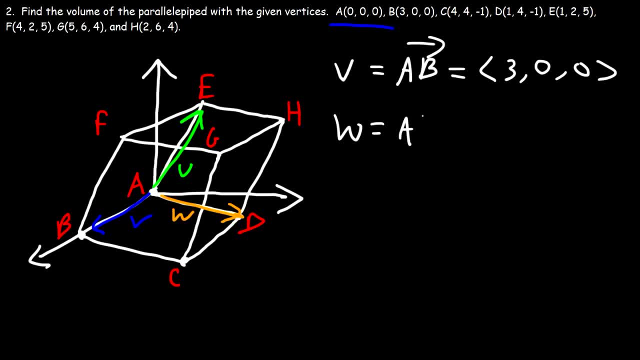 vector W, which starts from A and points towards D, And so if we subtract D from A, it's just going to be the same as point D. get the vector 1,, 4,, negative 1.. And the last one, vector u, which is the same as vector a, e. 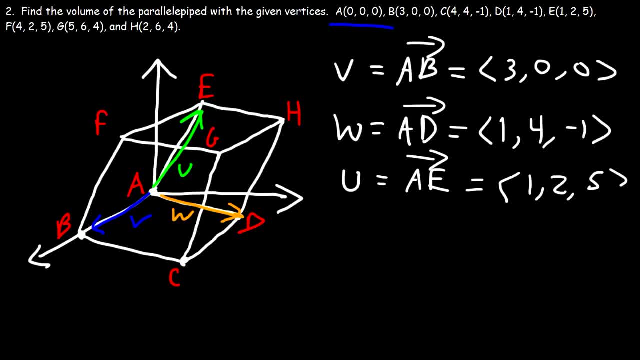 That's going to be 1,, 2, and 5.. So now that we have these three vectors, we can calculate the triple scalar product to get the volume. So the volume of the parallelepiped is going to equal the vector u times or the dot product of vector u and the cross product. 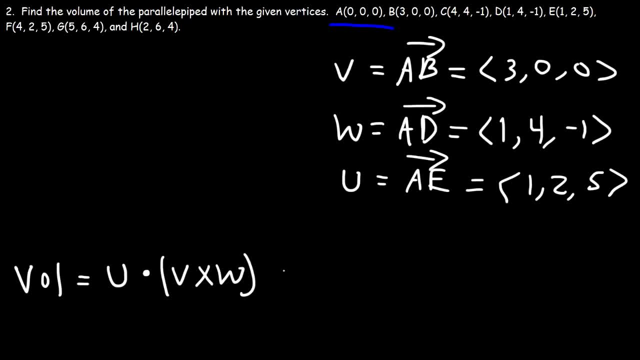 of vectors v and w. So now let's turn this into a 3 by 3 matrix. So let's start with vector u, which is 1,, 2,, 5.. Next we have vector v, which is 3,. 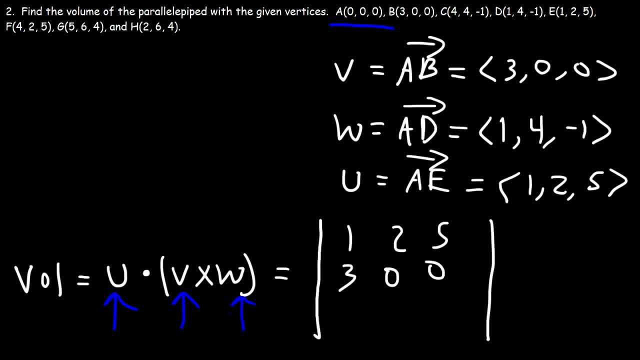 0, 0.. And finally vector w, and that's 1, 4, negative 1.. So let's start with the first number in the first row, So it's going to be 1, and then that number is in the first row, first column. 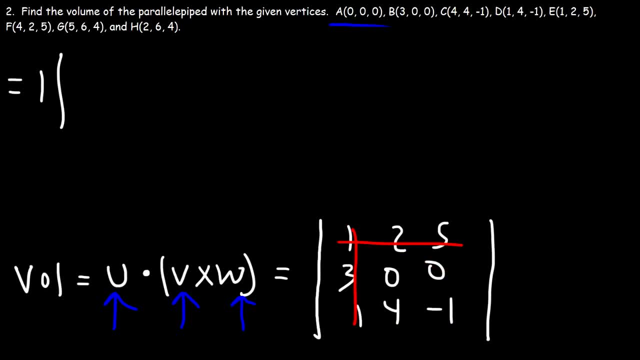 leaving behind a 2 by 2 matrix: 0, 0, 4, negative 1.. Now the next number in the first row is 2, but we need to put a negative sign in front of that And that number is in the first row, second column. 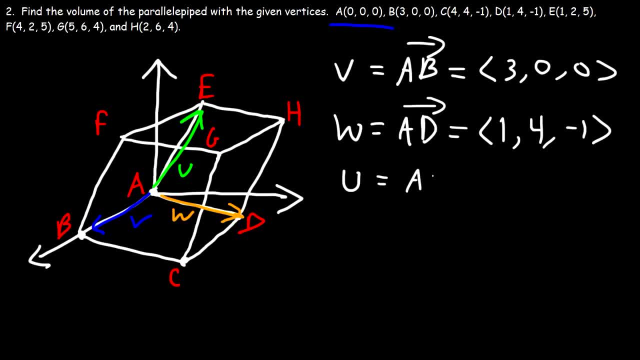 one, vector U, which is the same as vector A, E, that's going to be 1,, 2, and 5.. So now that we have these three vectors, we can calculate the triple scalar product to get the volume, So the volume of the parallelepiped. 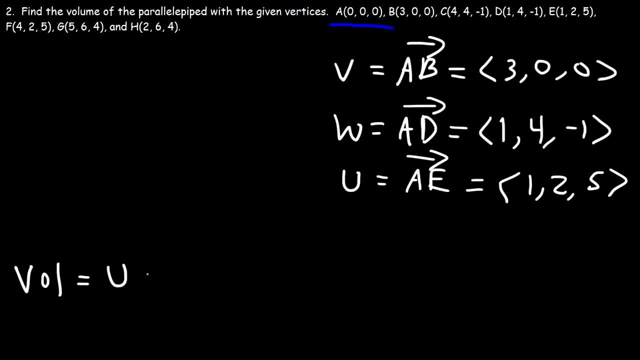 is going to equal the vector U times, or the dot product of vector U and the cross product of vectors V and W. So now let's turn this into a 3 by 3 matrix. So let's start with vector U, which is 1,, 2,, 5.. Next we have vector V, which is 3,. 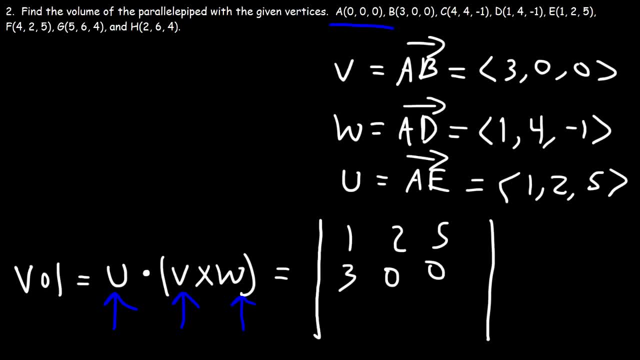 0, 0.. And finally, vector W, and that's 1, 4, negative 1.. So let's start with the first number in the first row, So it's going to be 1, and then that number is in the first. 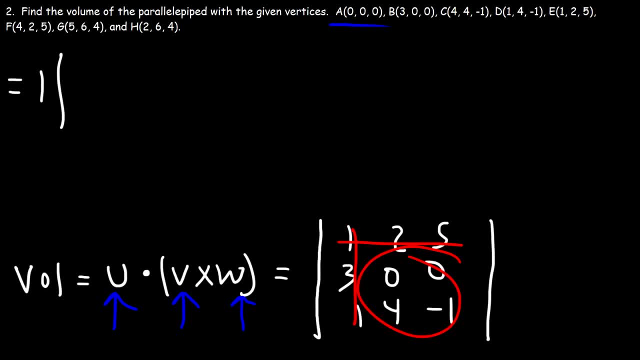 row first column, leaving behind a 2 by 2 matrix: 0,, 0,, 4, negative 1.. Now the next number in the first row is 2,, but we need to put a negative sign in front of that. 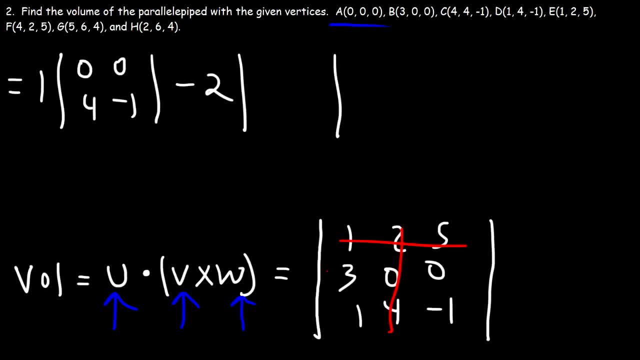 And that number is in the first row, second column, leaving behind the numbers 3, 1, 0, negative 1.. Now the last number in the first row is 5 and that is in the first row, third column. 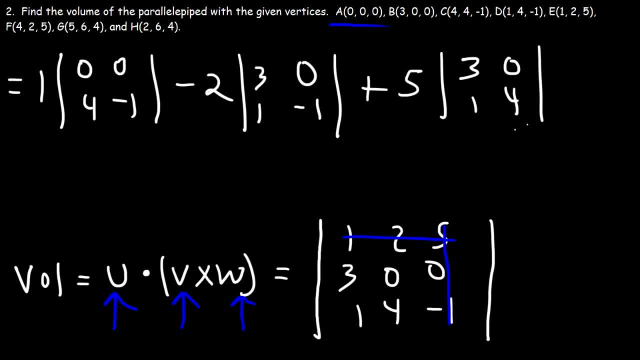 And so we have left over 3, 0, 1, negative 1.. So we need to put a negative sign in front of that: 0, 1, 4.. So this is going to be 1 times 0 times negative. 1 is 0, minus 0 times 4, which 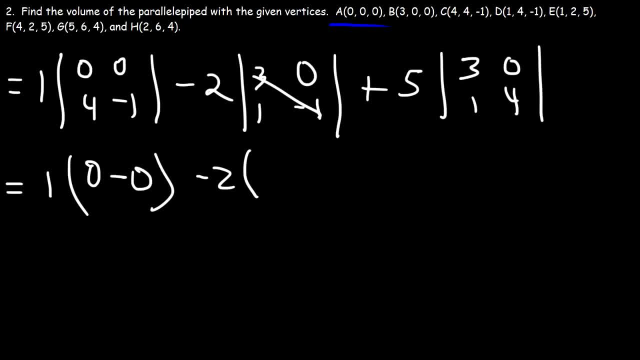 is also 0.. And then here we have 3 times negative 1, which is negative. 3, 0 times 1 is 0, and then 3 times 4 is 12, minus 1 times 0, which is 0. So this whole thing is 0.